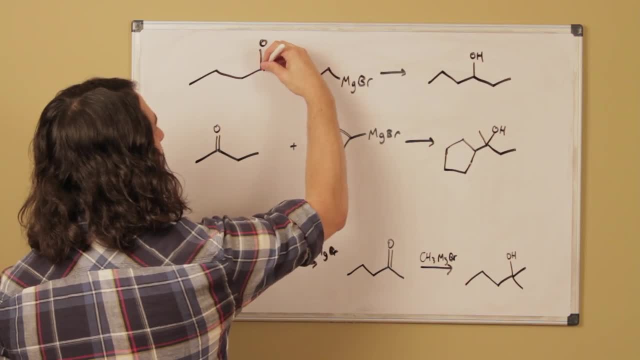 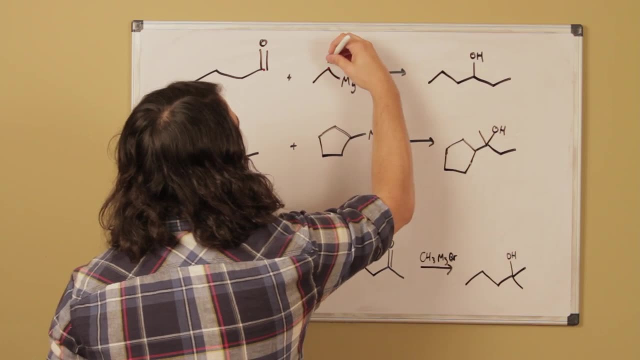 the carbon that is attached to the magnesium and the carbonyl carbon on the magnesium, on the substrate, that are going to generate a new carbon-carbon bond. this is because the insertion of the magnesium atom into the carbon-bromine bond reverses that polarity. 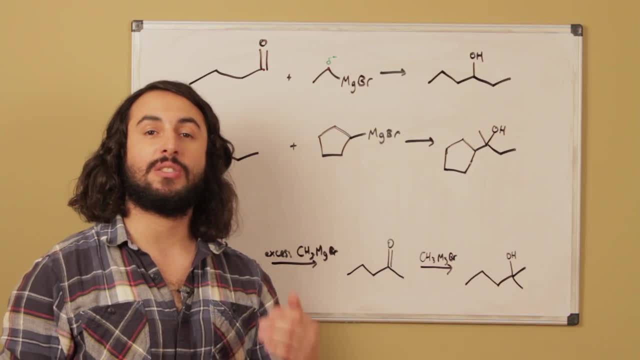 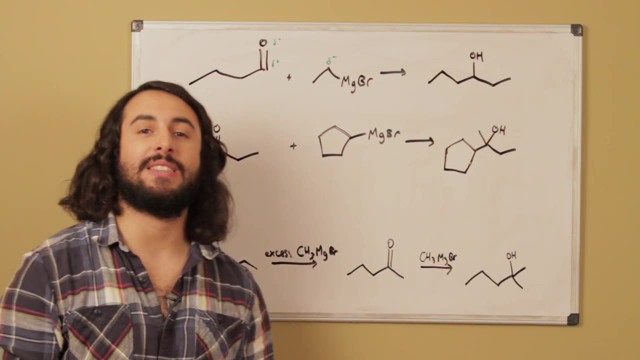 we're going to have a partially negatively charged carbon atom, so that is a source of nucleophilic carbon. and then, once again, we know that a carbonyl looks like that. we've got a partially positive carbon. a carbonyl carbon is partially positive, so any reaction? 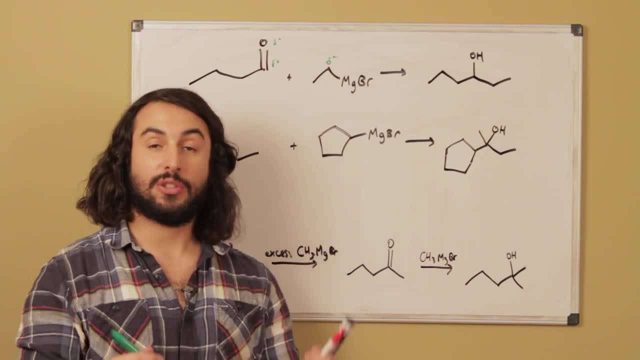 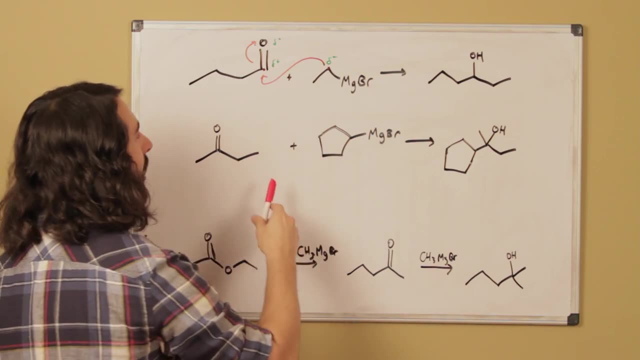 in chemistry is always electron excess meets electron negative, so we're going to have electron deficiency. so that's how grignard reactions work. so in this case we know that this carbon is going to go ahead and attack there. pop that up a little bit of acidic. 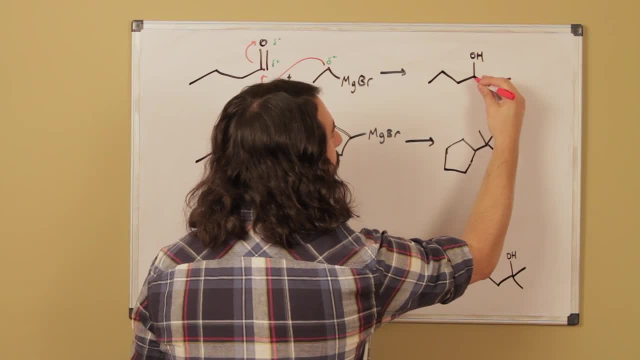 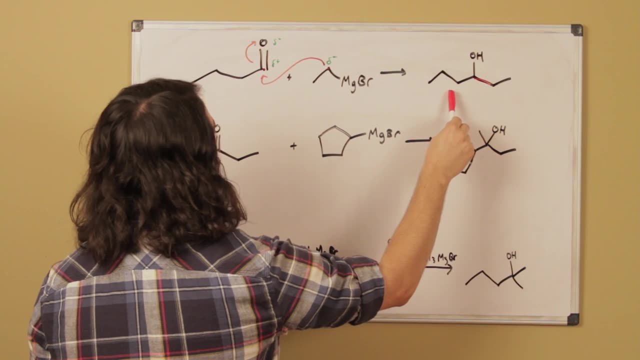 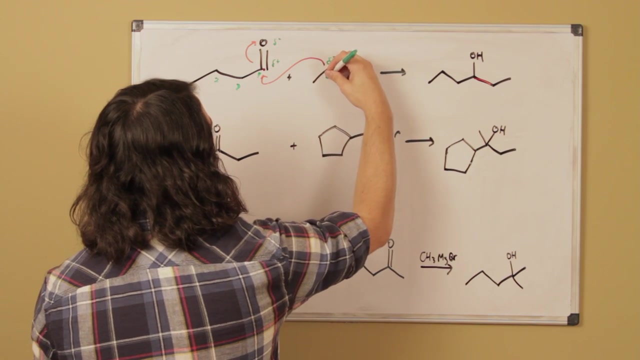 workup and we'll get the alcohol. so this is the new bond that we have formed right there. these two carbons came from the grignard reagent and these four were already there, so let's number them: 1, 2, 3, 4, and then this is going to be 5 and 6. 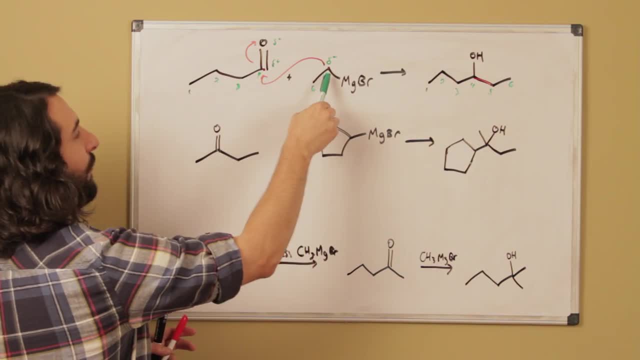 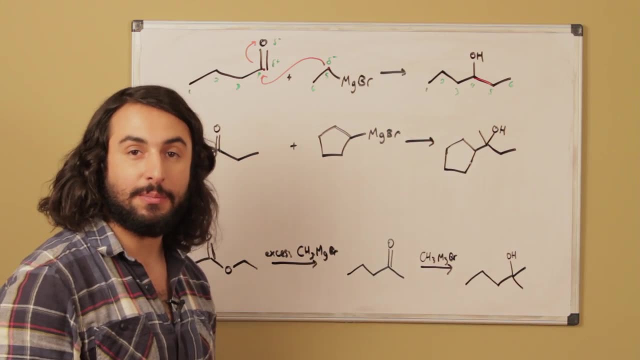 1, 2, 4, three, four, five and six. so five from the Grignard reagent, the one that was nucleophilic, and four the carbonyl carbon, now have that new bond between them. so remember that is. 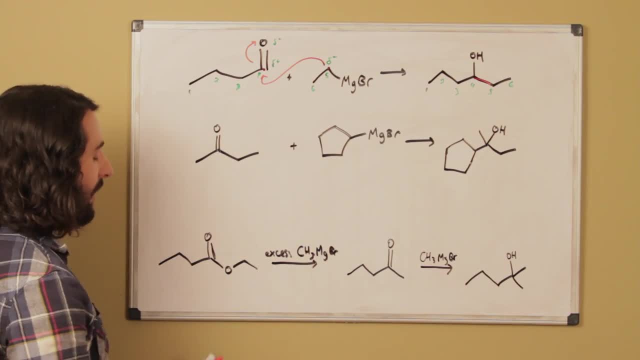 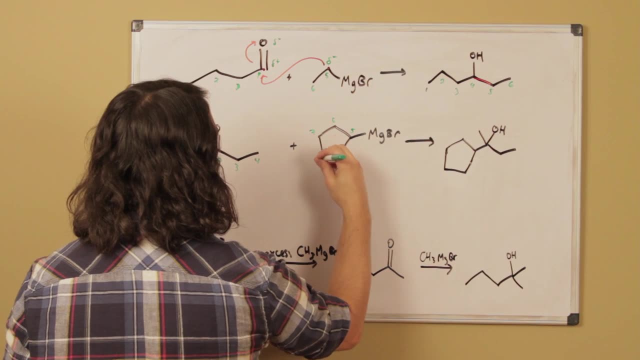 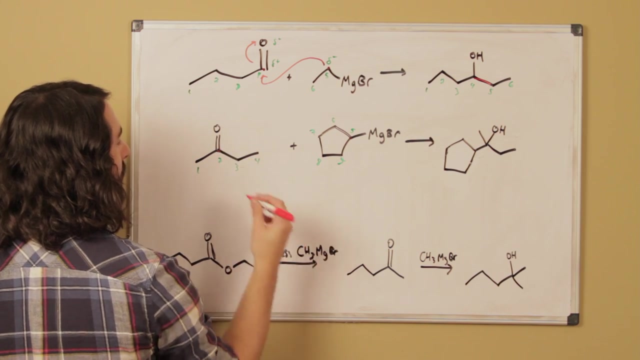 always going to be the case for Grignard reactions. now, once again right here. let's number these: one, two, three, four, and then we've got five, six, seven, eight, nine. it is going to be once again. this is the carbon that is connected to magnesium. this is the. 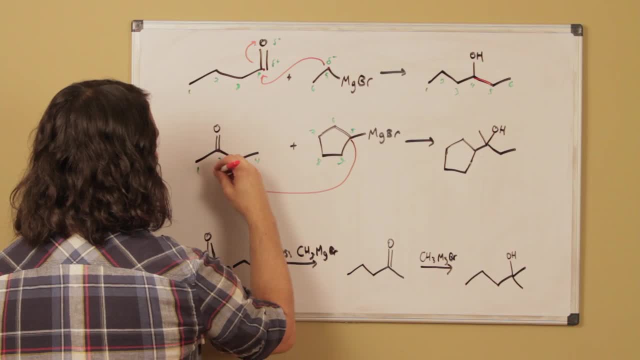 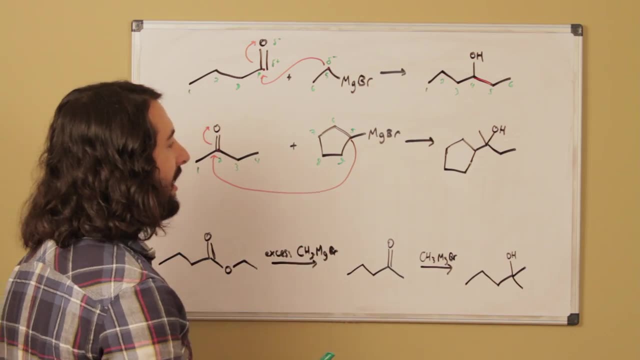 carbonyl carbon. you're going to have that attack here. pop that up, that'll get protonated upon workup and we've got our alcohol. so here we need to make that new bond, we need to show that new bond, but then a very common error is to create. 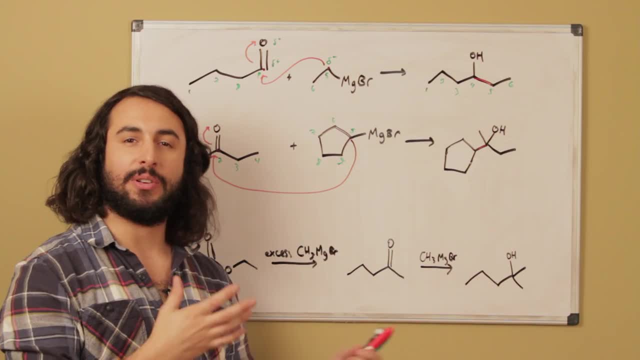 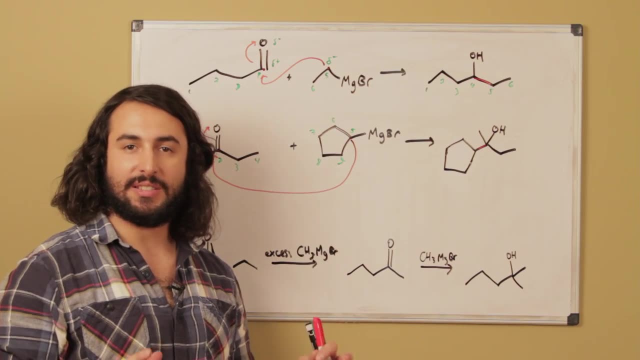 the correct connectivity, but then have something weird happen with the other carbons. remember that the only thing that has happened is a new bond between this carbon and this carbon. everything else that is there simply remains where it is, so that's why it's sometimes good to number our carbons like that we know. 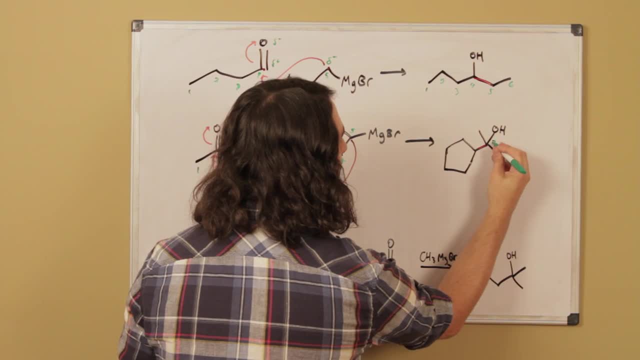 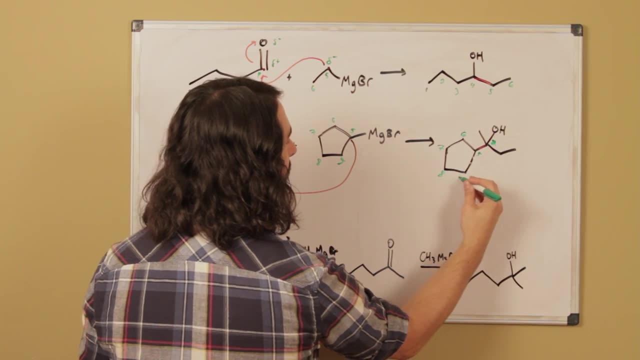 that we've made a bond between two and five, so there's five, or, sorry, there's two and here's five, and then let's number around the ring, like we had six, seven, eight, nine, and then, connected to carbon, two on this substrate was carbon. 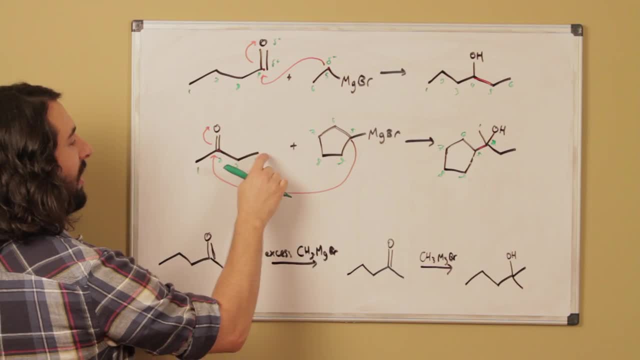 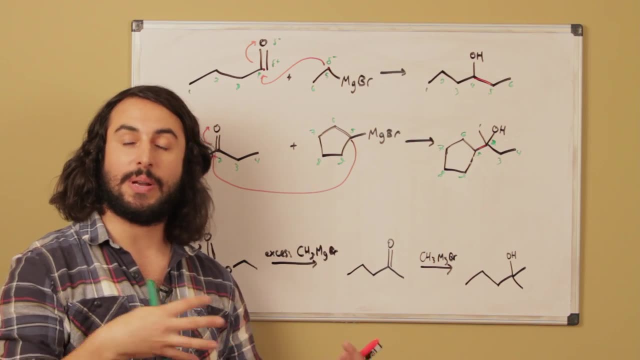 one, the methyl. so that's still there, nothing happened to that. and then three and four, right there, those are still there, nothing happened to those. so if you're having a difficult time visualizing the transformation itself, usually you can number the carbons and then, if you just say to: 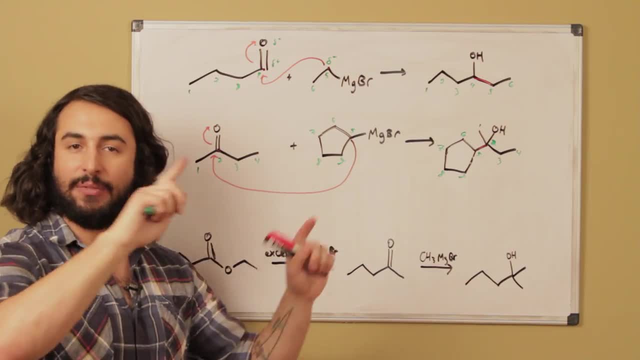 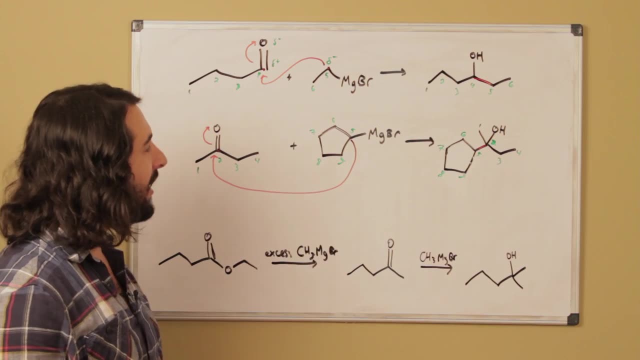 yourself five and two. there's a new bond there, and then everything else that those were connected to they're still connected to. so two, there's one, three and four, etc. so there's our product for that one. now, this one's a little bit different because we have an ester substrate and 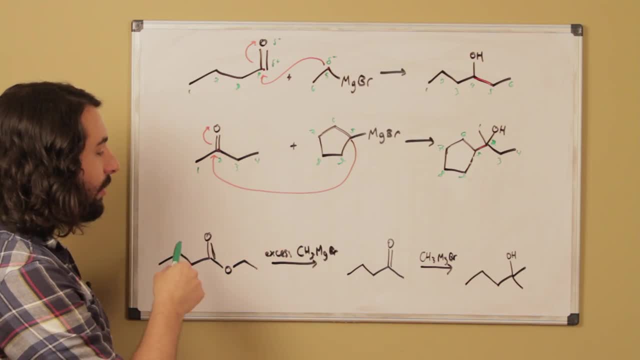 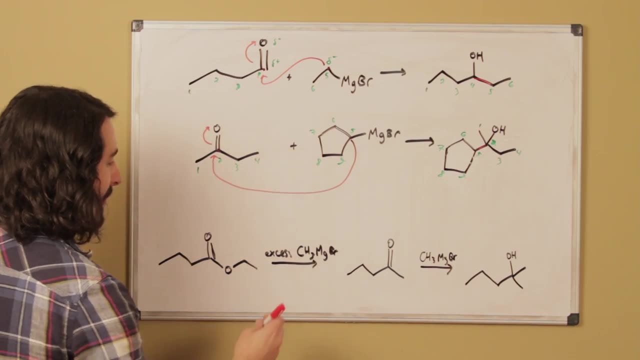 if you recall from my Grignard lecture, we know that an ester substrate in the presence of excess Grignard reagent can undergo two consecutive Grignard reactions. because what happens is: so this is all we have, is this methyl here, so that is going to attack, that can go up there. 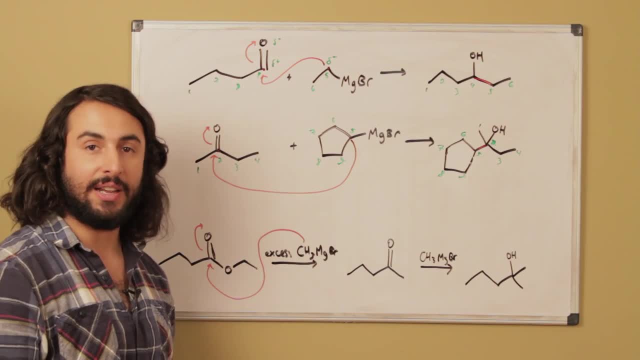 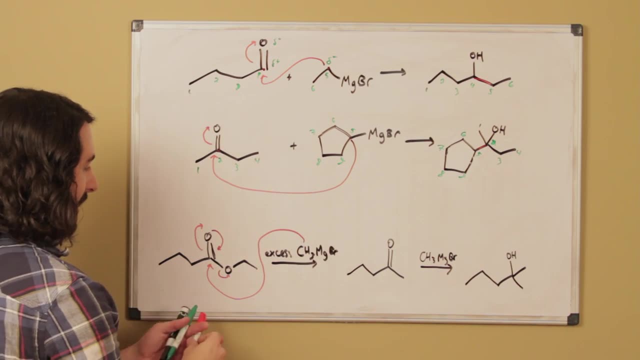 and then we get the oxyanion, but then, instead of protonating, this can actually come back down and kick off the alkoxy group. so we have added our grignard, we have added our methyl grignard reagent. right there, that's the. 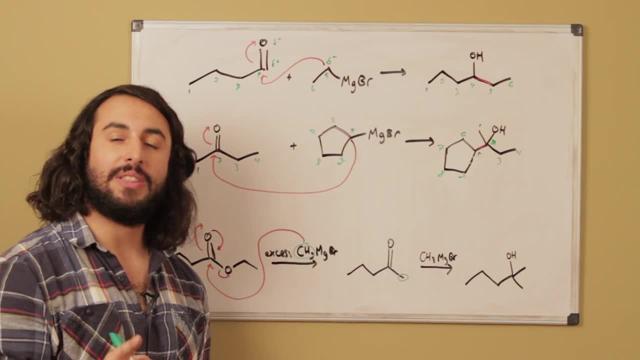 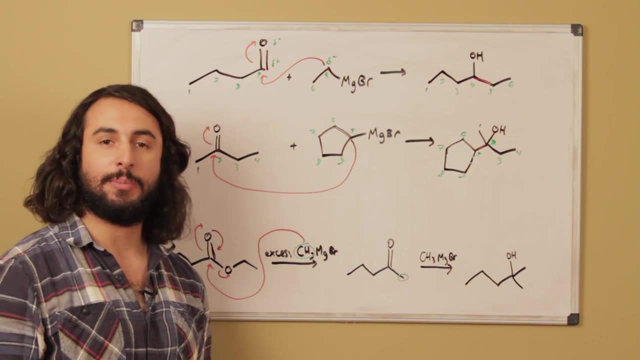 new methyl and we've kicked off that alkoxy. but in kicking off the alkoxy group we regenerated the carbonyl and we know that any ketone or aldehyde is susceptible to attack from a grignard reagent. so if we have excess grignard, 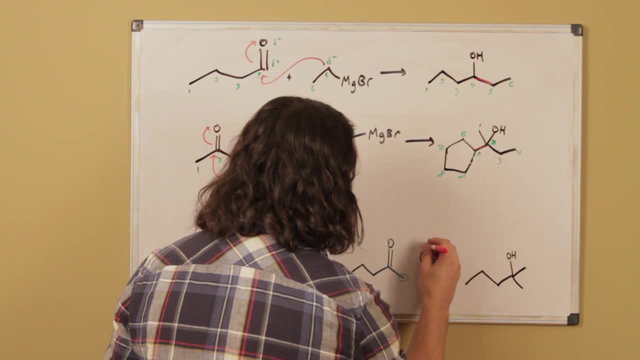 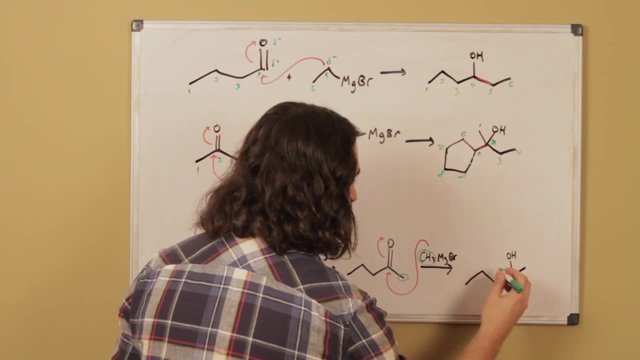 reagent, at least two equivalents. that means that we can do this again. another grignard reagent that's swimming around can find that ketone, and now, all of a sudden, we have added another methyl grignard reagent, and so what we can see? 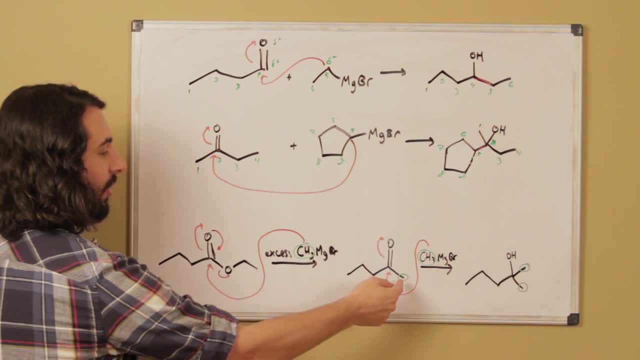 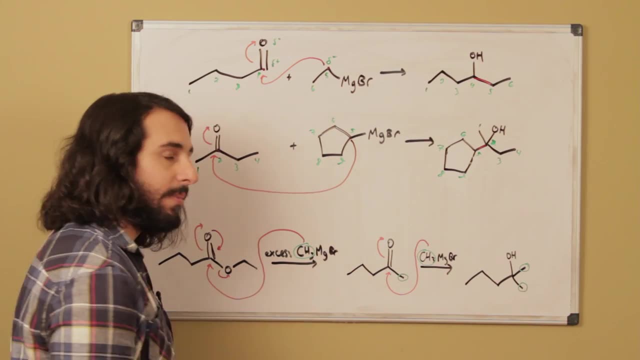 here is by kicking off the alkoxy group, we regenerated the carbonyl. there's one equivalent of our, of our grignard reagent, and then we can go ahead and do it a second time, because that carbonyl was regenerated and we've got.